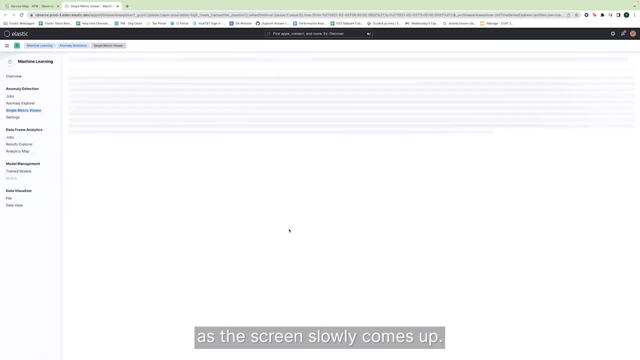 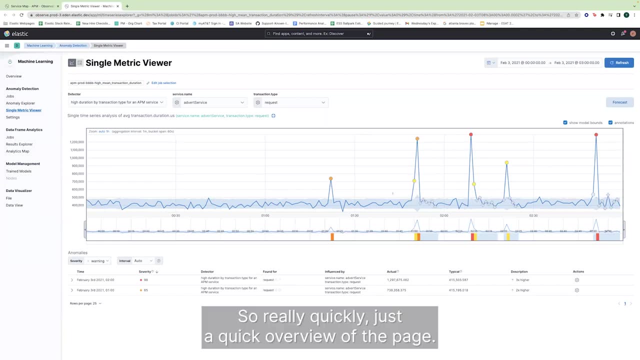 As we click on this anomaly, as we see here, as the screen slowly comes up, we see we have a few different anomalies coming out of the norm. So really quickly, just a quick overview of the page. The light blue shading here indicates the typical expected behavior and this is based on our unsupervised non-detection, just learning the typical patterns of your systems. 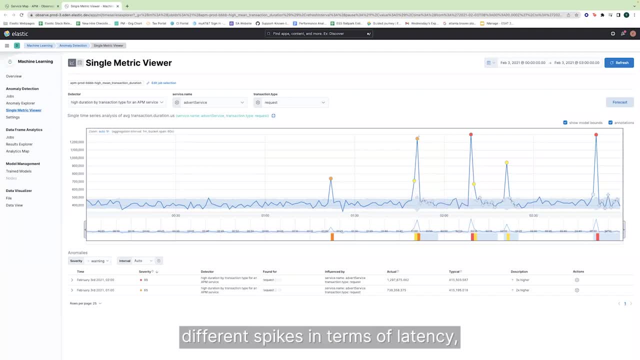 As you can also see, we've had a couple different spikes in terms of latency, but we didn't get alerted on them, The reason being we've specifically defined the alert condition to only alert us via Slack on critical anomalies. And speaking of critical anomalies, let's go ahead and take a look at this. 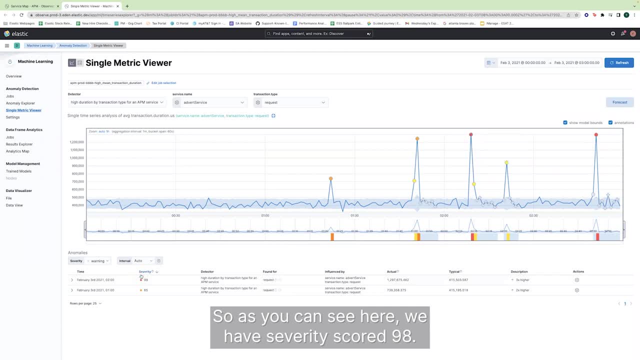 We'll look at the one we got alerted on. So, as you can see, here we have a severity score of 98.. The detector kind of gives us some information on what it's detecting and, more importantly, it gives us typical behavior and the actual behavior and, more importantly, how far out of bounds that typically is. 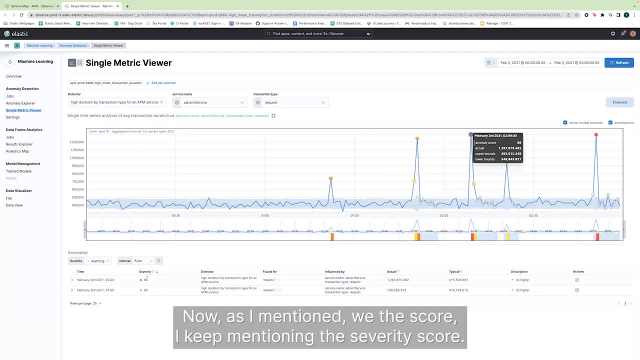 Now, as I mentioned the score, I keep mentioning the severity score. So, as part of our objective to operationalize data science, we don't want to always just tell you what is anomalous, right. As you can see, we've had anomalies throughout the system, but we've only been alert on the critical one. 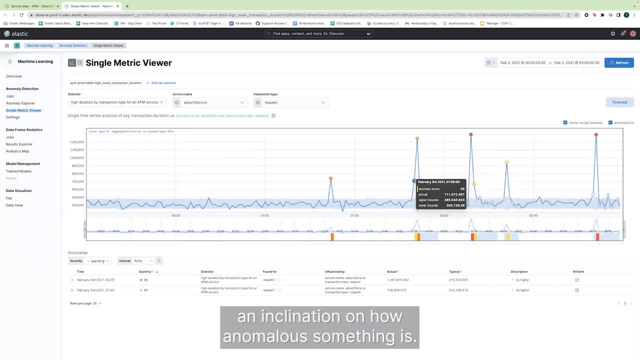 And that's because we want to be able to give you just an inclination on how anomalous something is, so that way you can go ahead and determine your workflow, so that way you're not constantly getting pinged for these lower-level anomalies which may just be, you know. 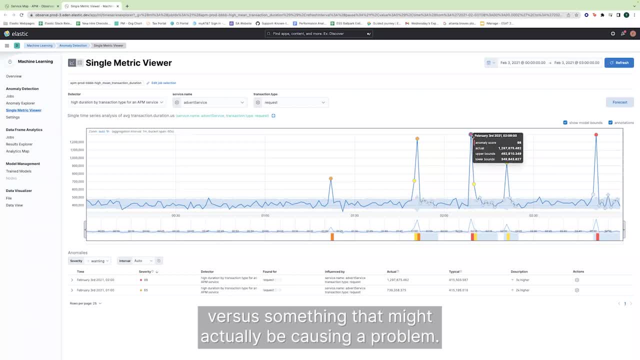 typical every now and then, a small latency spike versus something that might actually be causing a problem. As nice as this anomaly is, it just lets me know that I have high latency in my application, which is great. It's nice that I'm alerted before my customers are letting me know there's an issue, but it's not really helping me truly understand what may be causing the issue. 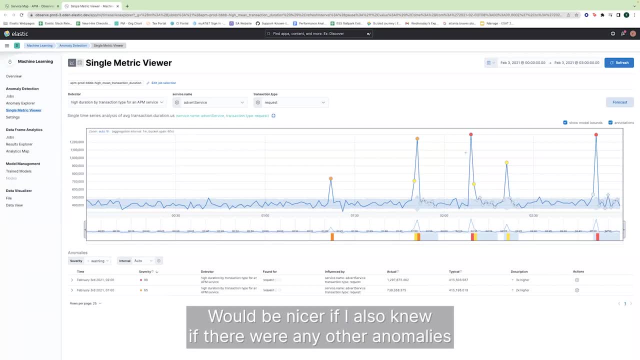 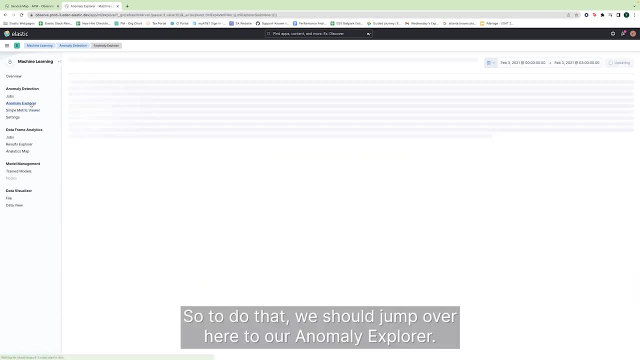 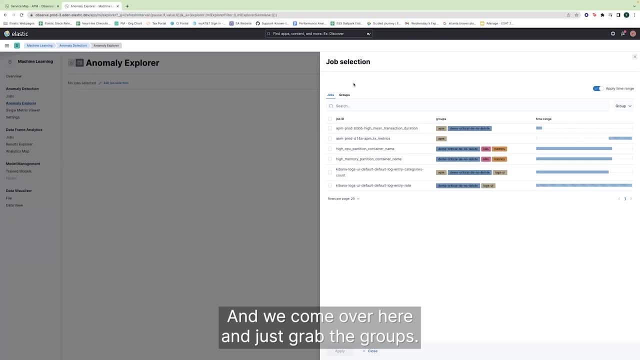 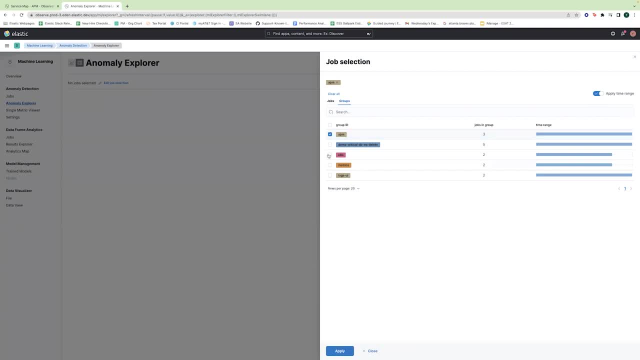 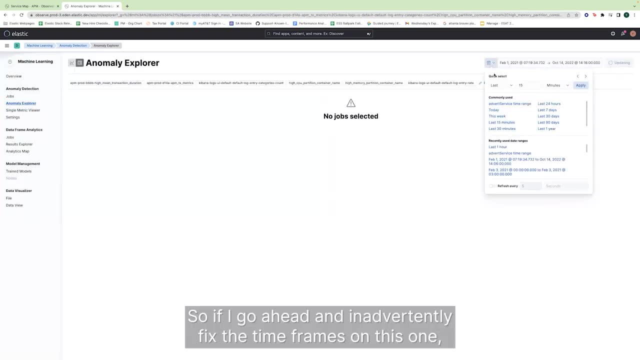 And in this case I want to look at the APM anomalies, any anomalies in my Kubernetes infrastructure and also in my logs. So if I go ahead and inadvertently fix the time range on this one, we can see a few different anomalies. 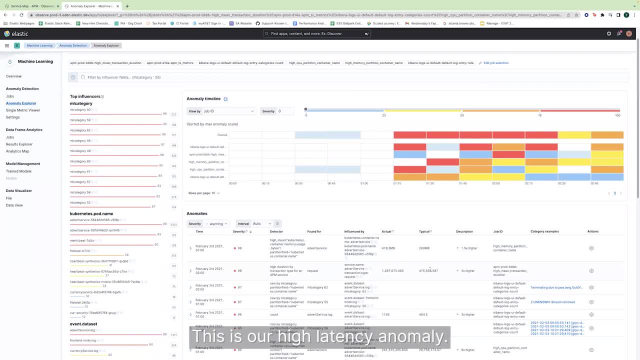 But what we're also seeing is our original anomaly. right, This is our high latency anomaly. But then what we're also seeing for the advert service is we're also seeing a higher-than-usual memory utilization in the underlying container that's running the advert service. 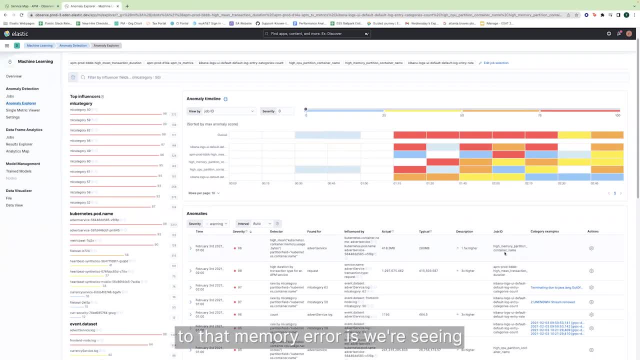 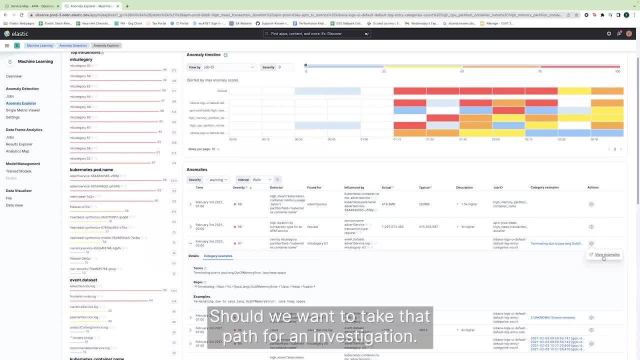 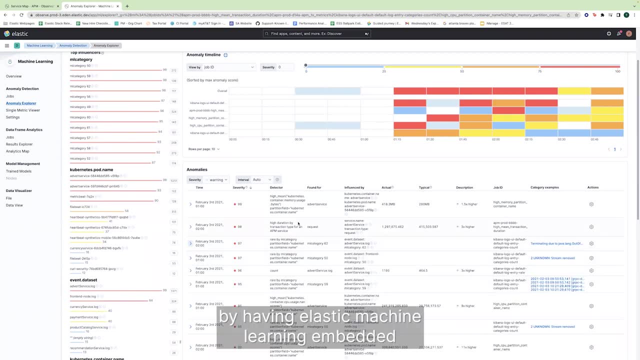 But, more importantly, what we're also seeing is we're seeing a rare log message for our advert service indicating an out-of-memory error. instances of where we're seeing the out-of-memory error should we want to take that path for an investigation. But, as you can see very quickly by having Elastic's machine learning embedded. 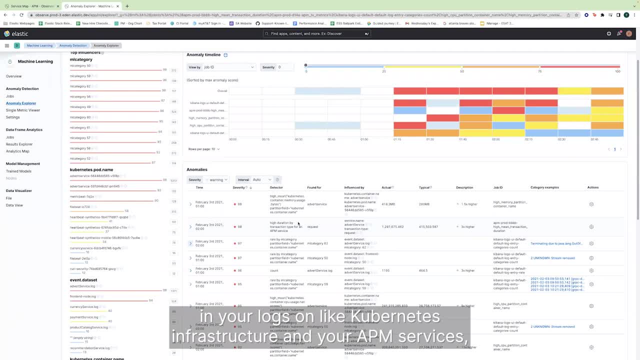 in your logs underlying Kubernetes, infrastructure and your APM services, you're not only able to indicate when you're having high latency, but you're also able to quickly and automatically surface other problems throughout your system that may indicate what's affecting one service. 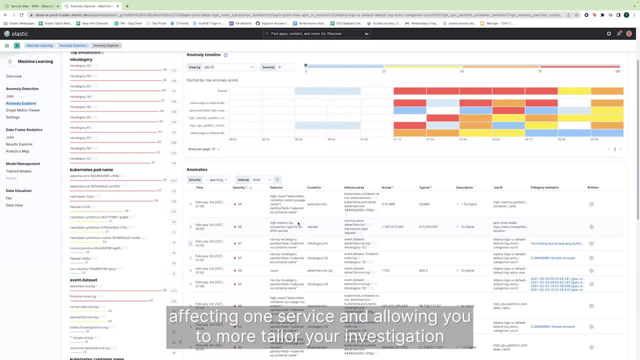 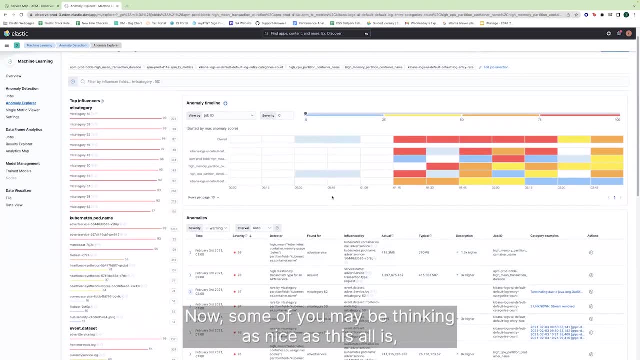 and allowing you to more tailor your investigation, and thus your resolution, in a more timely fashion. Now some of you may be thinking: as nice as this all is, this is a demo environment and you clearly have everything set up, So I'm going to go ahead and